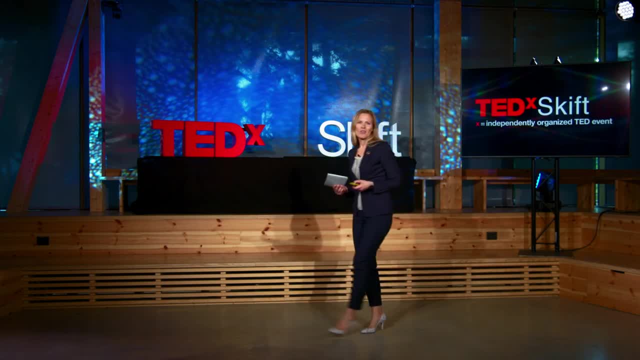 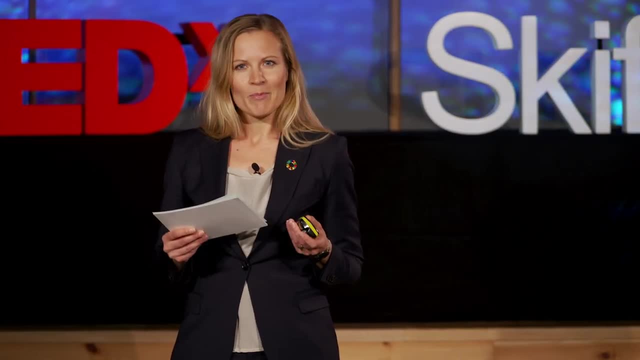 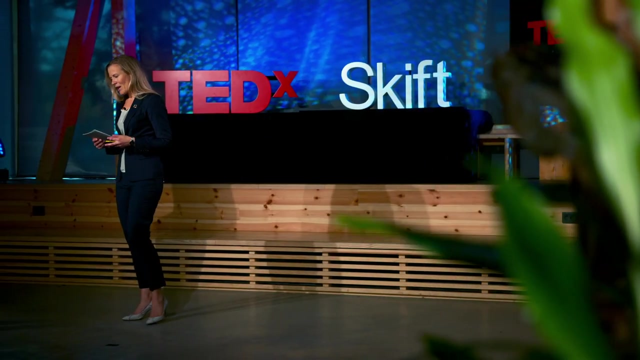 It is possible. in fact, This is the case with our investments in renewable energy in developing countries, And that is very good news, because we need to turn billions of investments into trillions in order to reach the goals in the Paris Agreement And what KLP has. 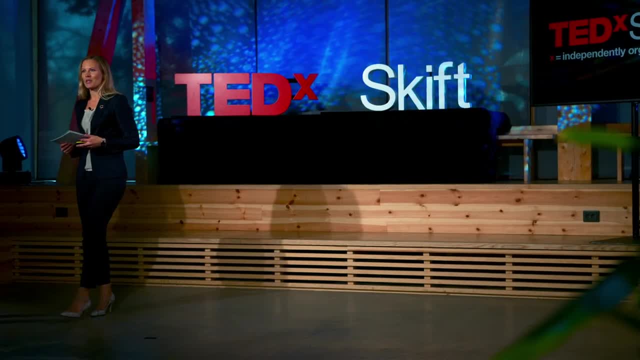 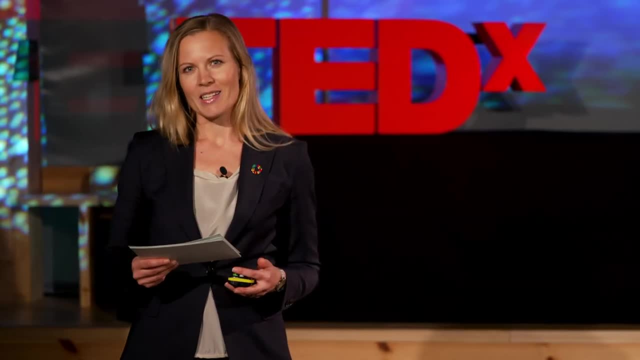 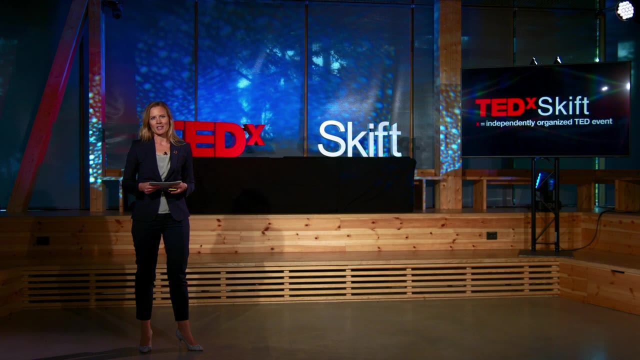 done can hopefully inspire other investors to do something similar. I'll share with you today the benefits of private sector investments going hand in hand with public sector investments, or blended finance as it is called. I want to show you some of the projects that we are proud. 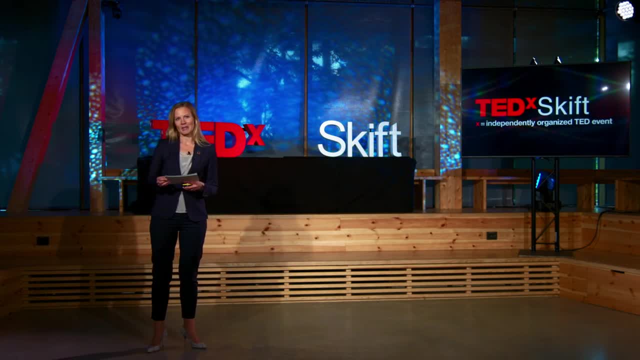 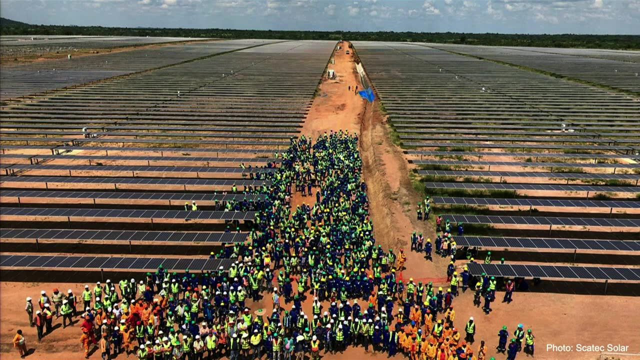 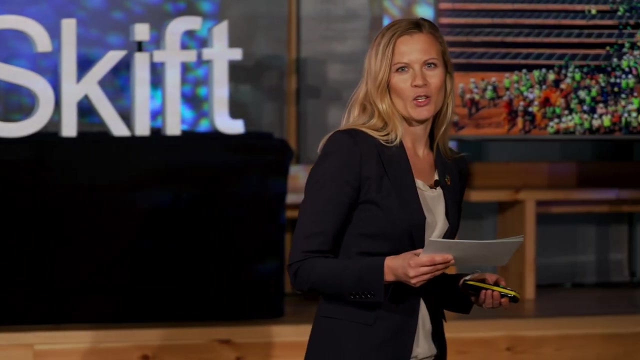 to be a part of. in order to describe the impacts of what we are doing, Let us start in Mozambique, which is one of the poorest countries in the world, where only 31% of the population have access to electricity. Here we helped finance Mokuba, Mozambique's first large-scale solar 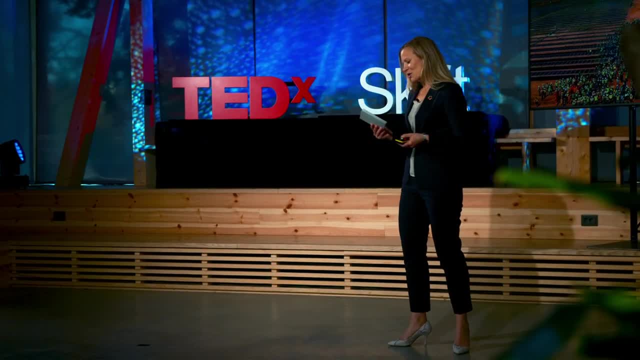 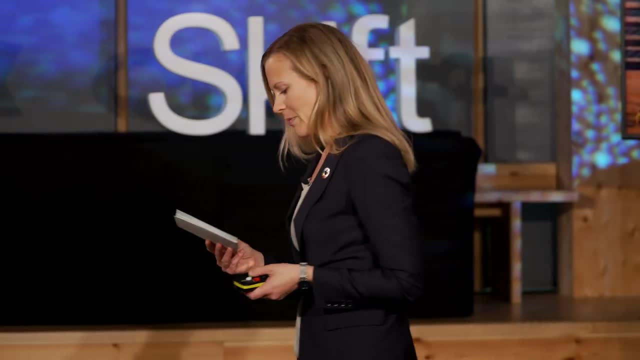 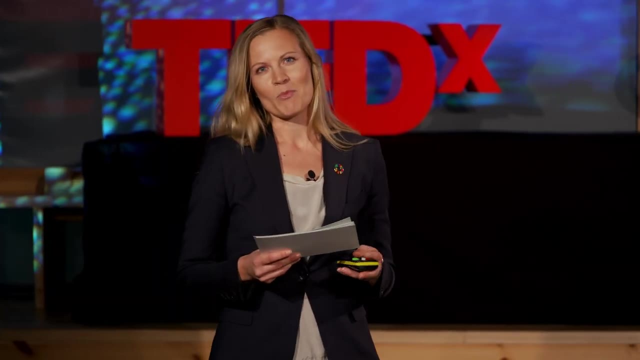 plant. It provides enough electricity to serve the equivalent of 175,000 households. Besides reducing emissions by around 80,000 tons annually, it helps to stabilize the grid and the energy supply in northern Mozambique. At the peak of construction, the project employed. 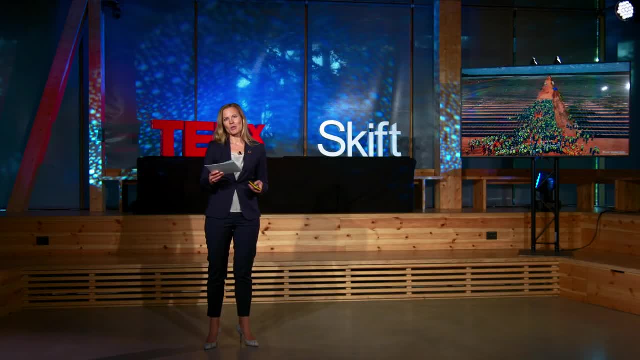 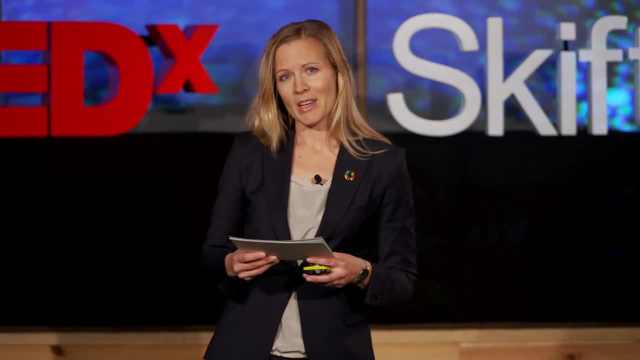 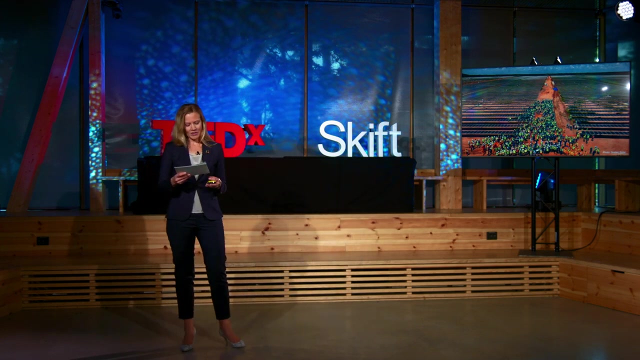 1,500 people, And although it currently employs only a handful of people, the wider impact on the economy is significant As people and businesses get a better, more stable access to energy, productivity improves and new businesses are established, leading to more jobs and economic growth. 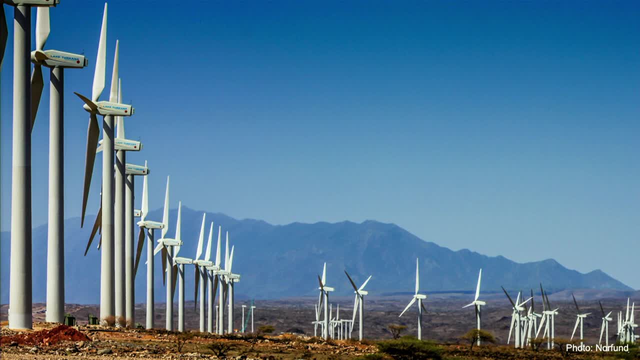 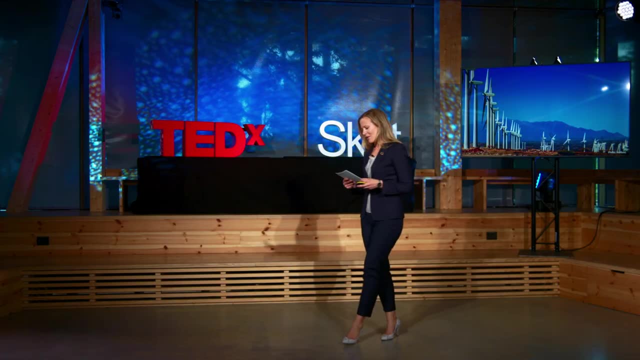 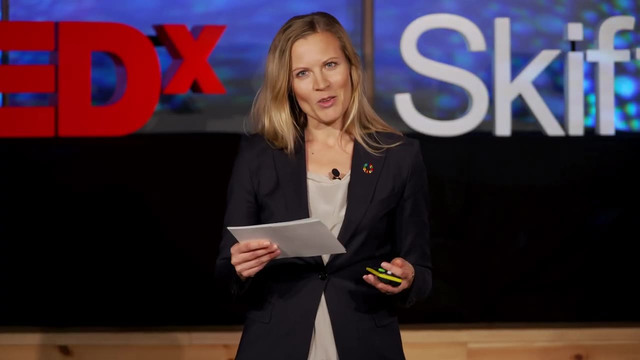 Now let us turn to the Lake Turkana wind farm in Kenya. This provides almost 17% of the area's total energy generation capacity, thereby avoiding production from fuel oil plants and providing reliable and low-cost electricity. This has also had additional positive impacts. 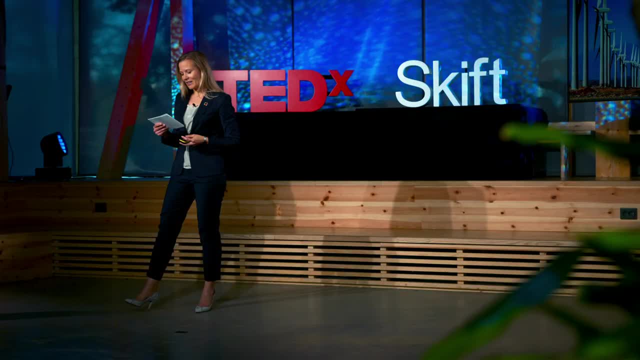 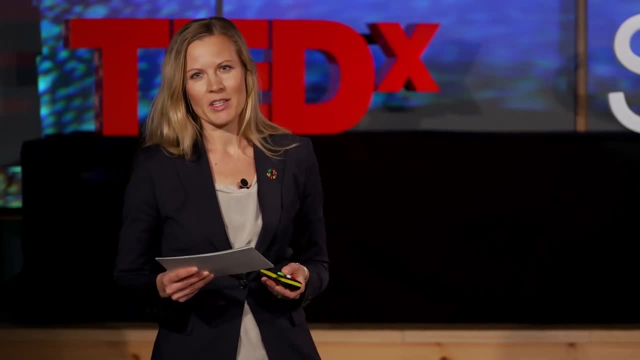 A new road has reduced time and costs of travel and has helped to increase trade in the region. These are investments that we have done with Norfund, the Norwegian investment fund for developing countries. We have started an investment company together with the Northland Fund for development of new jobs. and the Northland Fund for development of new jobs. As a result, we have also created a new growth fund. We have started investment companies in the region, including the region in the north, in Budapest, and in the south, in Tunisia, in the northeastern part of the world and in the northern part of the world. 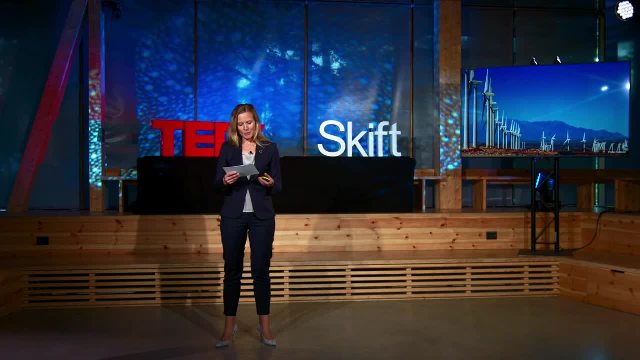 We have also started a joint venture fund under the name of Gioia Morgens for the growth of green私 and the Gioia Morgens in the north and southern part of the world start an investment company together which make direct investments in projects And although 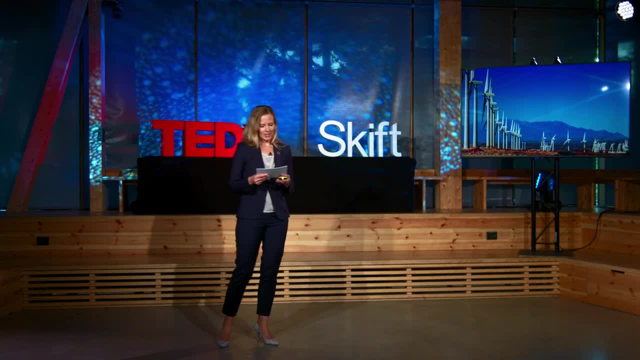 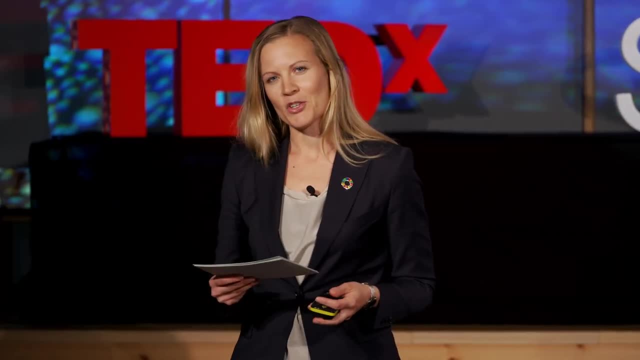 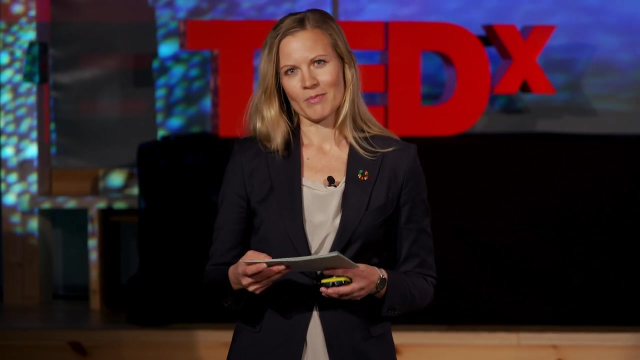 Norfund is publicly owned. it is commercially oriented And thanks to their expertise, operational setup and thanks to their way of structuring projects, KLP found a way to enter these markets that wasn't feasible before and wasn't feasible on our own. The return has also been attractive. 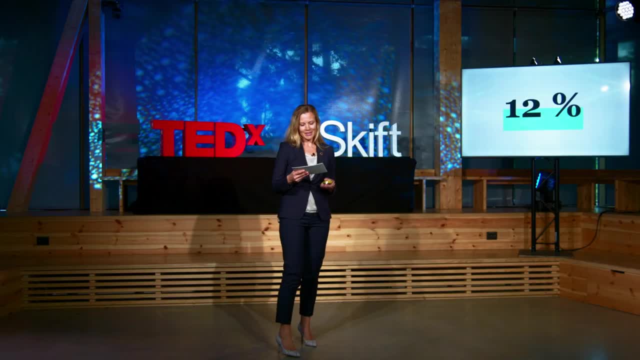 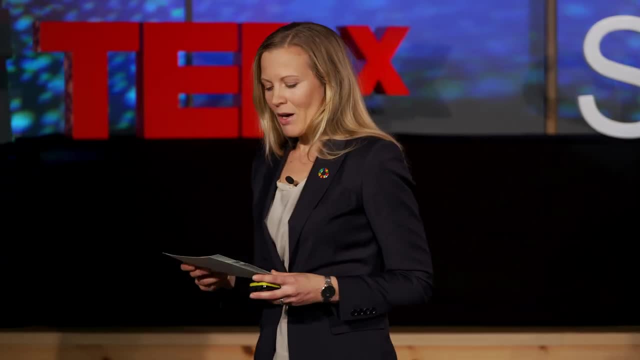 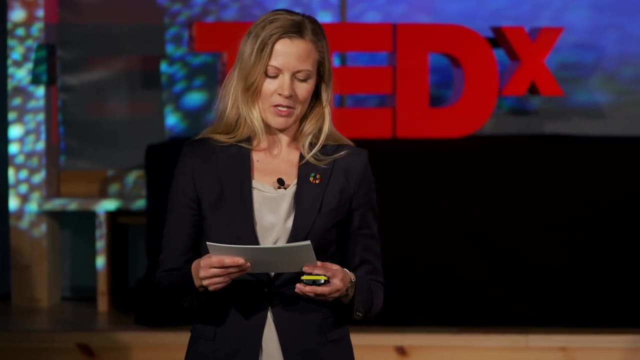 A 12% annual return so far. This has eased our initial hesitations and has encouraged us to continue building this portfolio. We all know that renewable energy plays a critical role in achieving the goal in the Paris Agreement. We must reduce the use of coal as an energy source. At KLP, we have already become coal-free and have focused more of our attention on the opportunities that come with it. According to the OECD, we need $6.9 trillion in infrastructure investments every year to 2030 to meet the goals of the Paris Agreement. Contrast this to about $300 billion, which is the figure 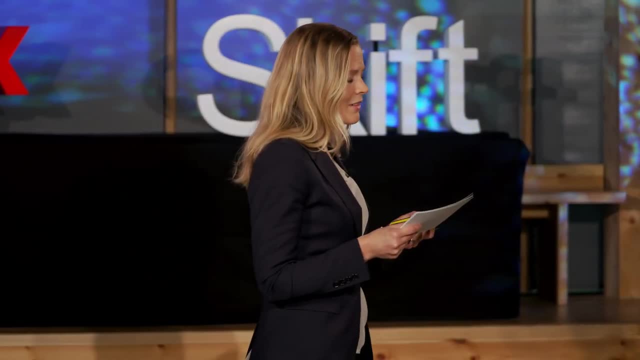 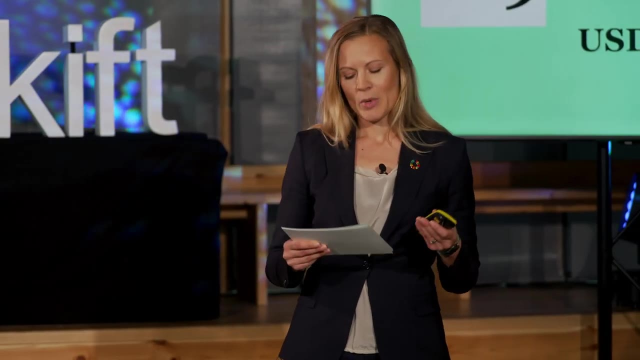 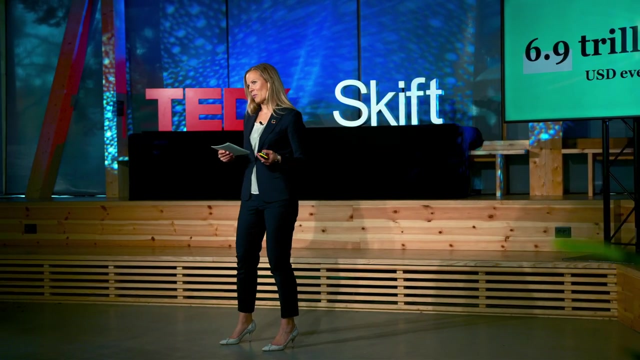 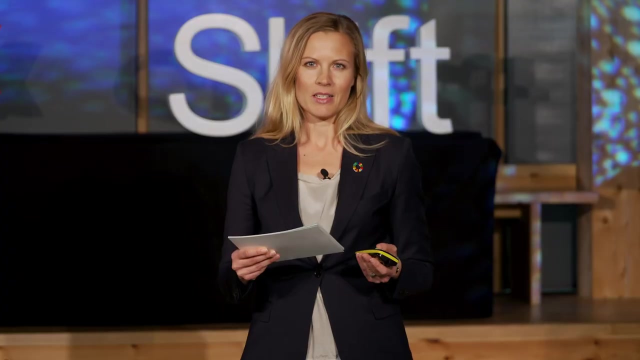 for the current annual investments in renewables. There is absolutely no doubt that we need more renewable energy, especially in developing countries, where we expect the largest amount of growth in needed capacity and where we now have the chance to replace the coal plants. The question is how this can be financed at the pace and the scale needed. 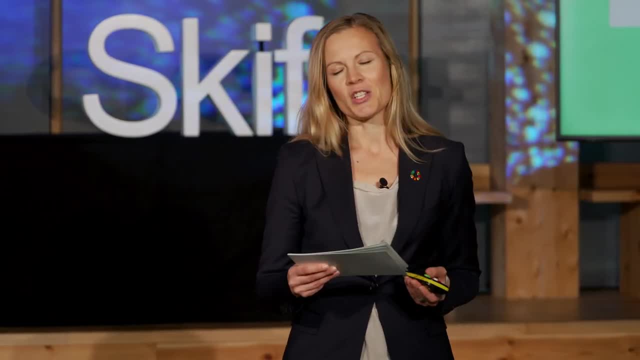 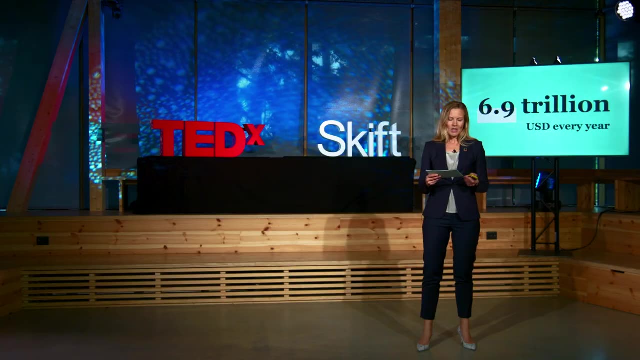 Again, we must turn billions into trillions in order to bridge the financing gap for renewables, And private institutional investors can and should take a bigger role. My message today is that KLP and other institutional investors can finance these projects as they in the future, But we also need to invest in renewable energy. 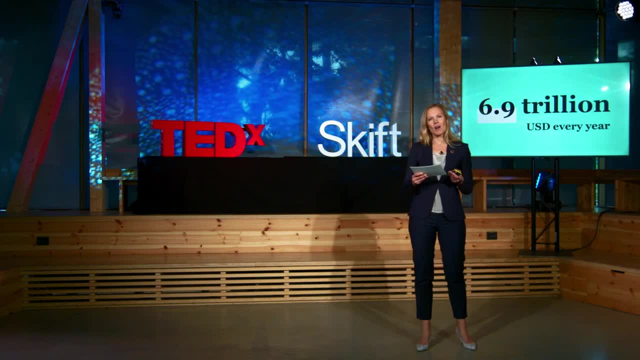 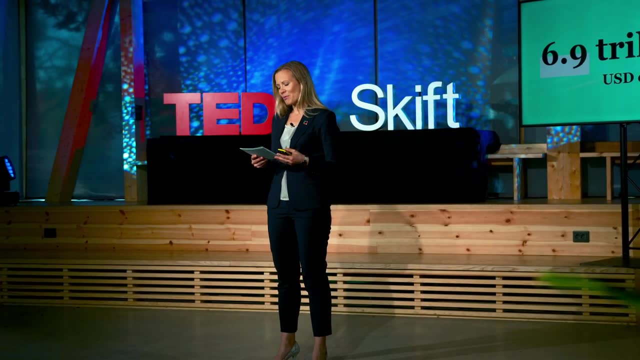 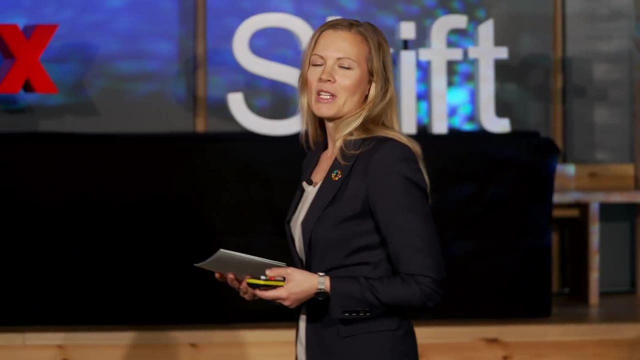 can fight climate change while, at the same time, harvesting competitive returns and managing the risks that are involved. By establishing new partnerships and using new tools, we can accelerate the spread of renewable energy. I already told you about KLP's and Norfin's co-investments. 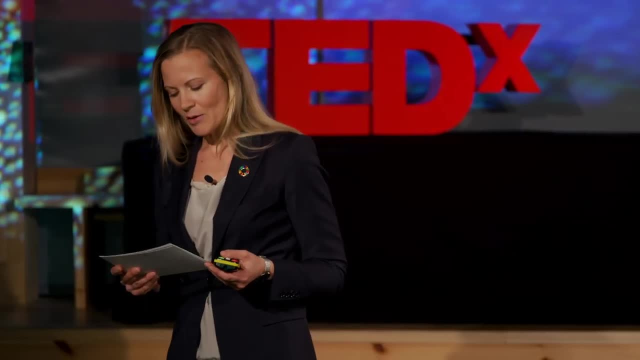 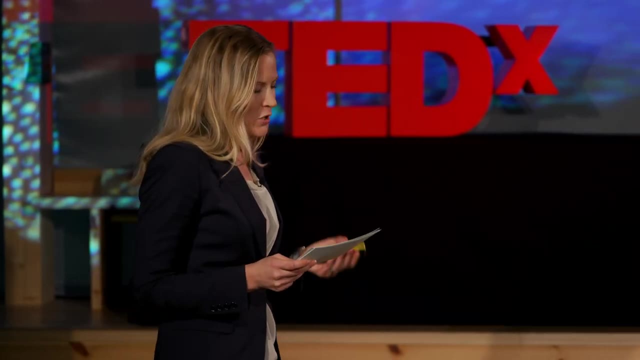 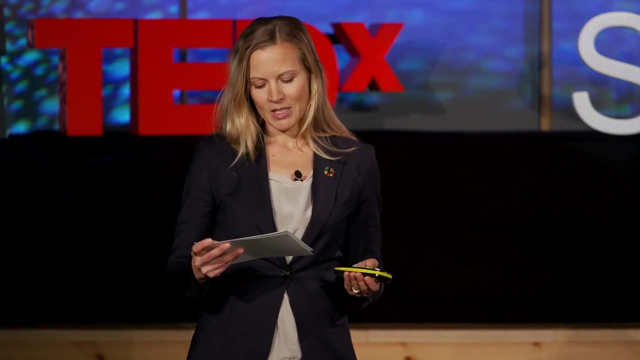 but there are also other ways that private and public investments can play together. Let's dig deeper in the blended finance toolbox. The beauty of blended finance is that both parties benefit. Public money can be used as an effective risk cushion, which means that investors dare to. 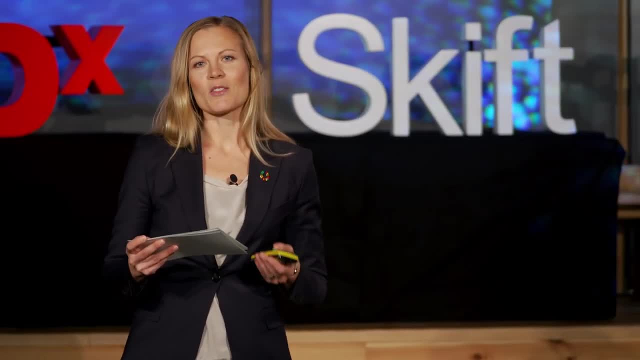 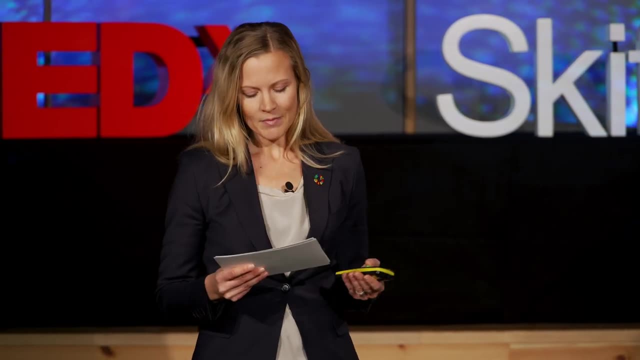 make investments that previously was too risky, as the risk is now lower. The government, on the other hand, can do more while spending less, as it becomes a catalyst for mobilizing private capital. The blended finance tool is a tool that can be used to make investments that previously was too risky, as the 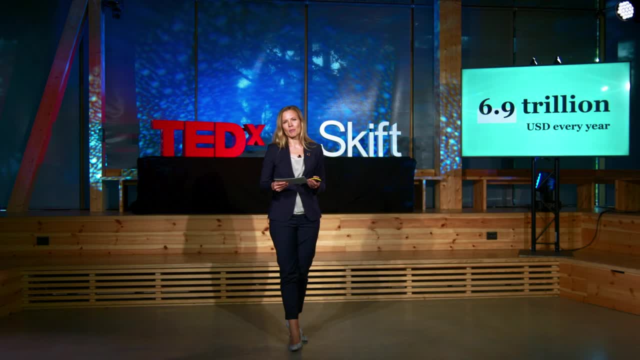 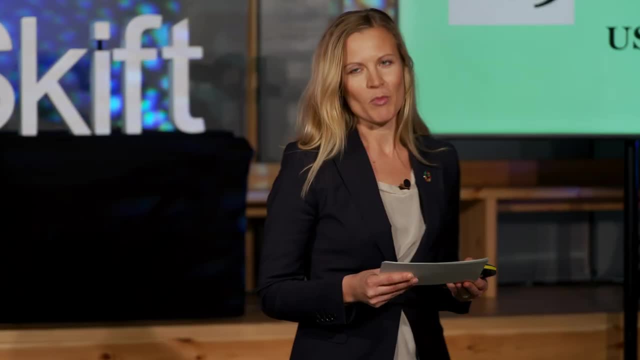 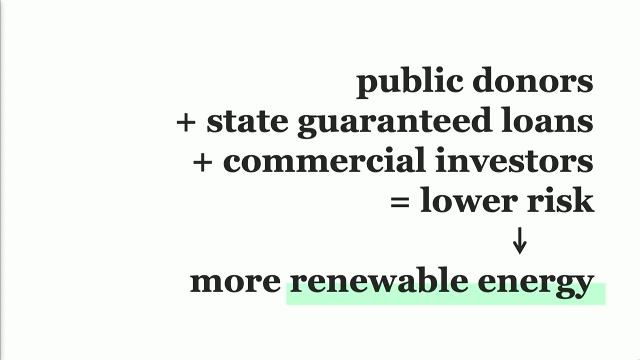 risk is now lower. The blended finance mechanisms have the potential to unlock private money that otherwise hadn't been there. It can be done in many ways, but I'll show you another example from KLP's investments. This is the innovative fund, Climate Investor, One that financed the whole life cycle. 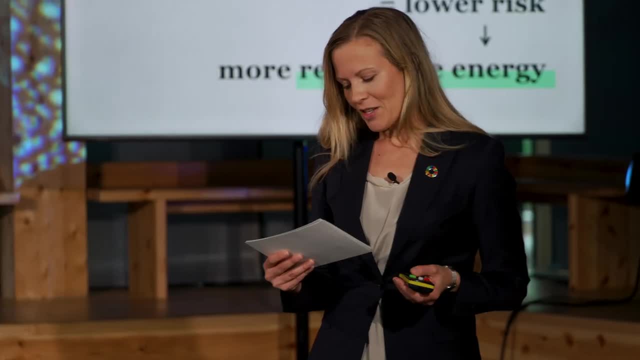 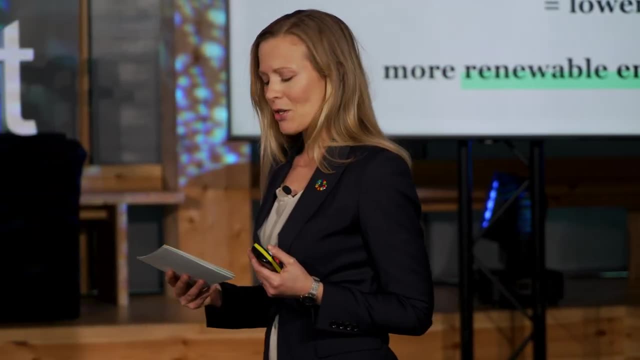 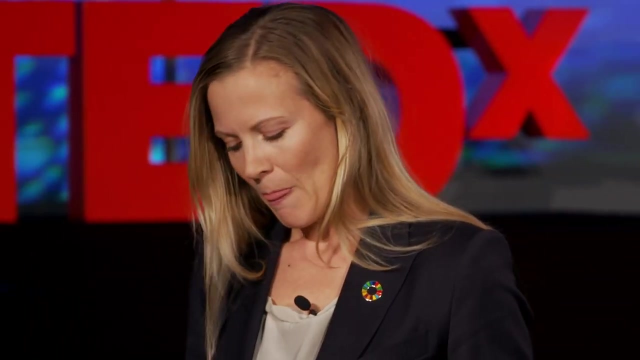 of a renewable project. This fund consists of several components, with three different financiers: Public donors, state guaranteed loans and commercial investors. The public donors are essentially giving a very cheap loan to the project. They are, however, the last ones to get their money back, meaning that in the case the project fails. 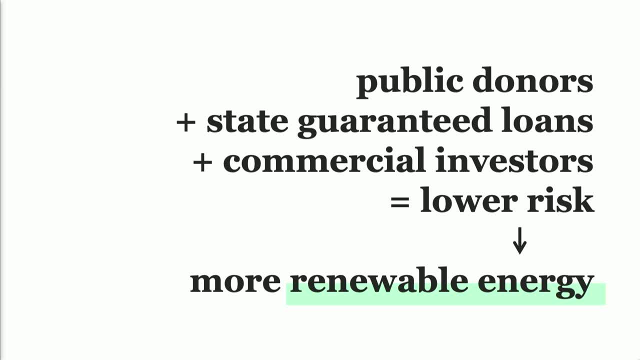 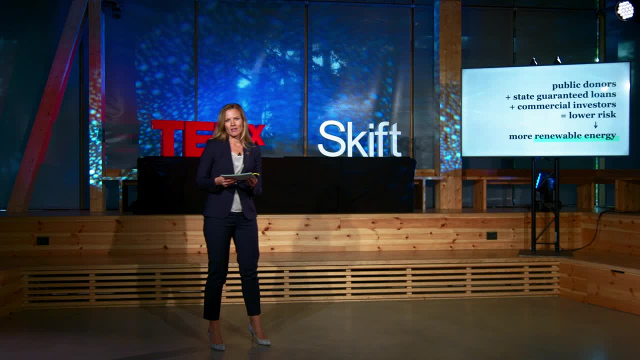 the initial loss will be covered by the donor. This is what is called a first loss mechanism. The state guaranteed loans help reduce the credit risk in the project and, combined with the first loss mechanism, it creates a risk and return profile that also fits a commercial and traditional pension fund like KLP. For KLP, blended finance has been a blessing. 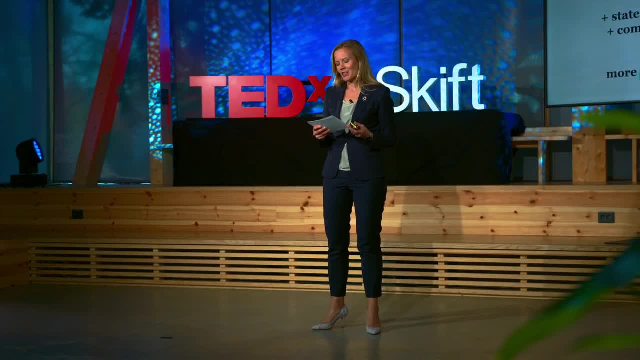 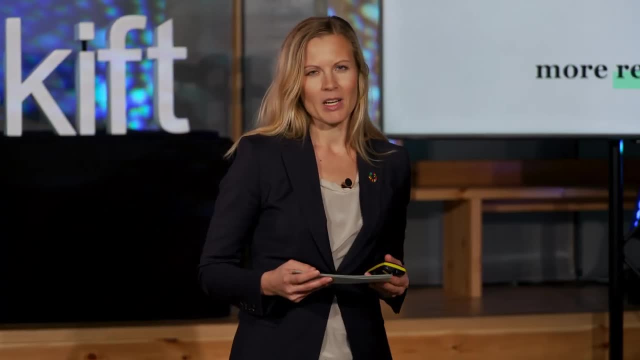 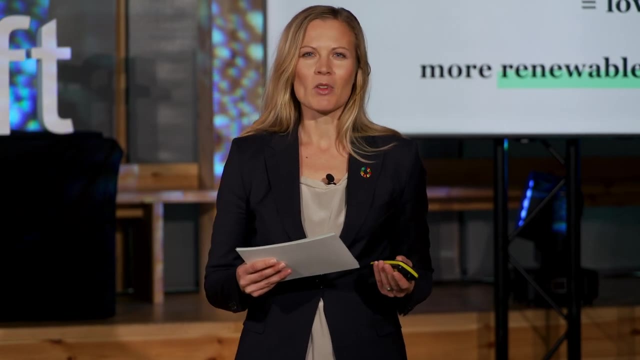 It lowers risk and we have found the operational partners that we need to do it. In short, it has given us the chance to get involved in these markets and directly in projects. It has created a win-win situation where we can ensure a responsible and sustainable management of pensions. 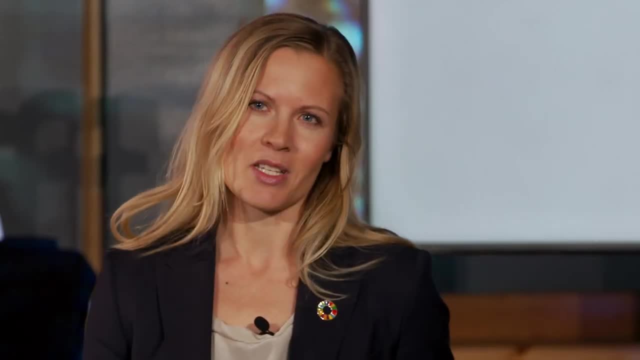 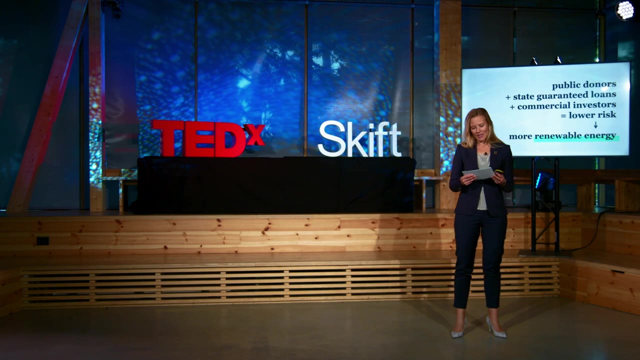 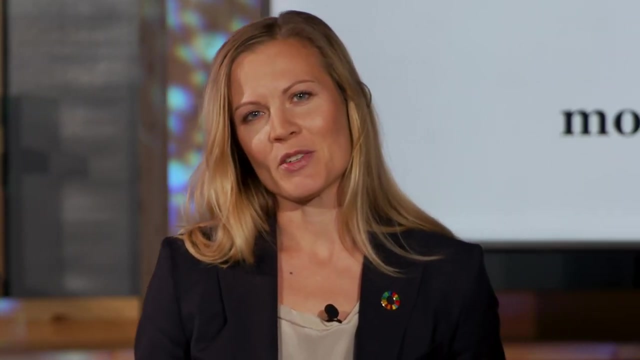 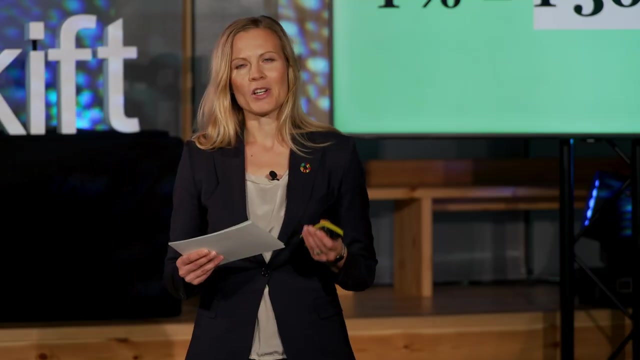 while at the same time, fighting change and having a positive impact on society. Institutional investors manage a vast sum of money. The asset owners that have signed the PRI, which is a network of investors and the world's leading proponent of responsible investing, control 90 trillion US dollars If these PRI asset owners were to direct 1%. 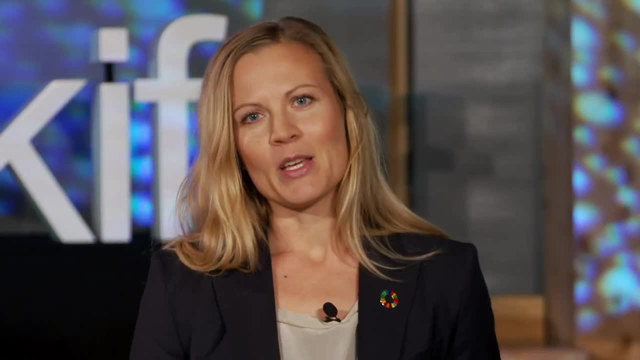 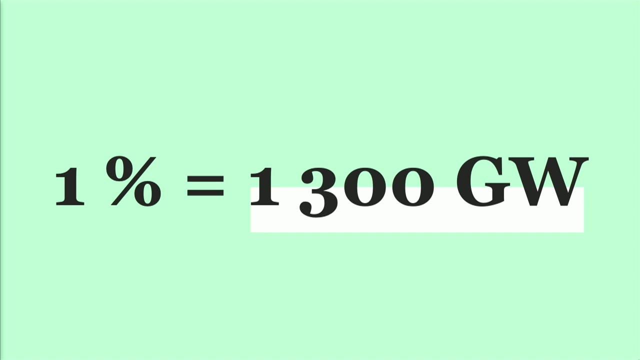 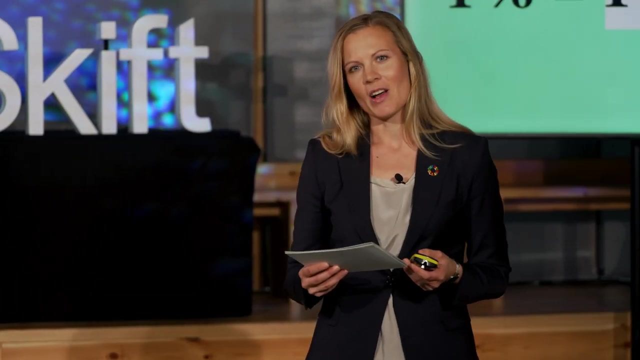 of their assets under management to renewable energy. this would mobilize financing of around 1,300 gigawatts of new capacity. That is over seven times more than what was installed last year. A recent article in The Economist shows that blended finance has struggled to grow despite its